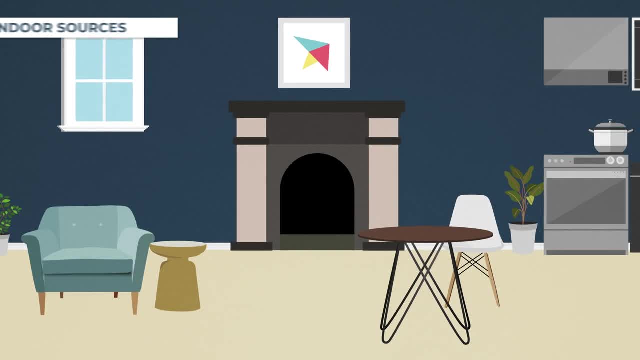 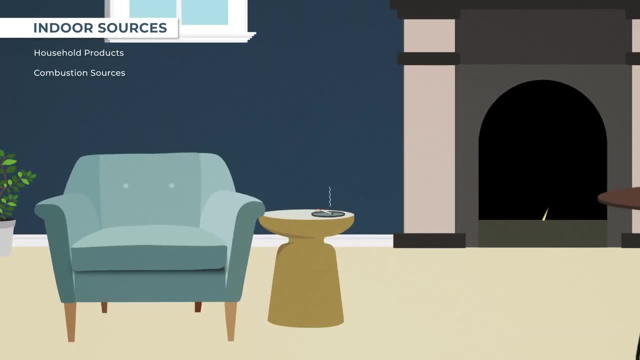 indoors from outside. Indoor sources include household products like cleaning supplies, insecticides and paints. Combustion sources like tobacco, fireplaces and cooking appliances are often found in buildings. In addition to the pollution sources, there are many other sources of air pollution. The most common sources are the air pollution. 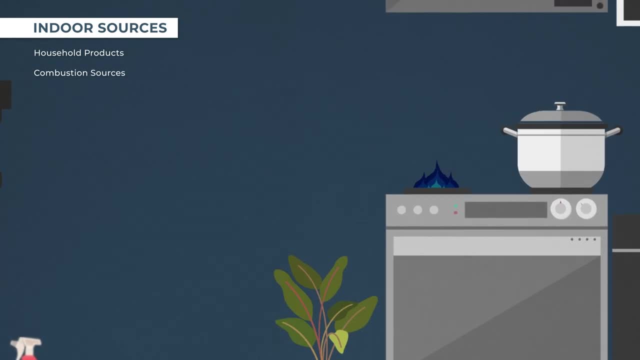 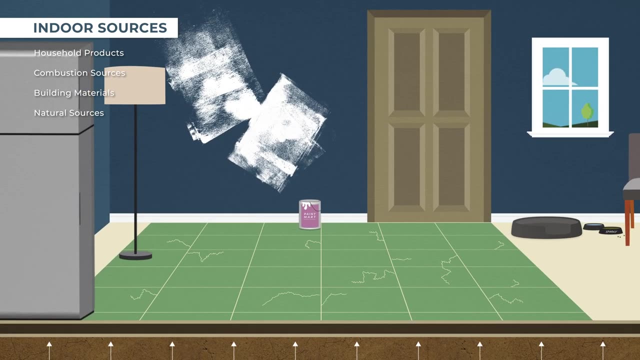 issues. These are often found in buildings, buildings and the environment. In these buildings, cooking appliances that let out carbon monoxide, old building materials and off-gassing chemicals from new building materials, natural sources such as radon, pet dander and mold. 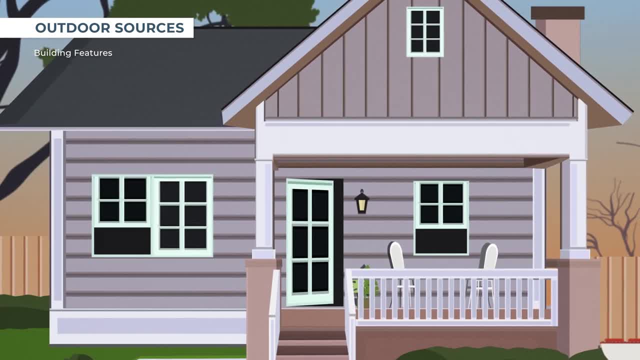 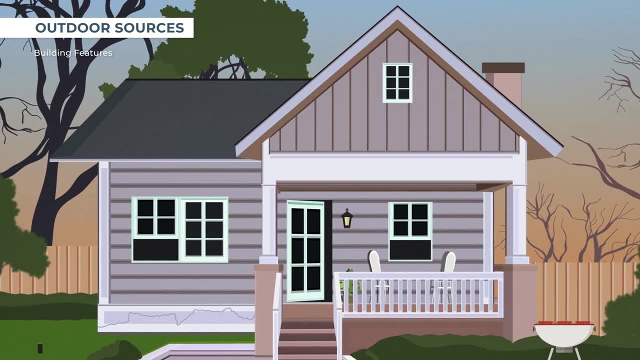 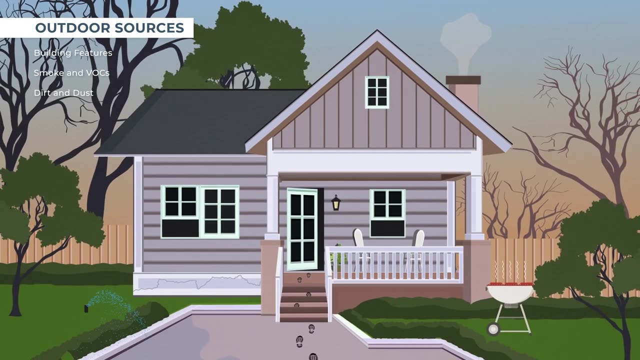 Outdoor sources can enter buildings through open windows, doors, ventilation systems and abnormalities in a building structure like a cracked wall or foundation. smoke from chimneys and VOCs from running water or cooking Dirt and dust left behind by shoes and clothing can be host for pollutants that adhere to. 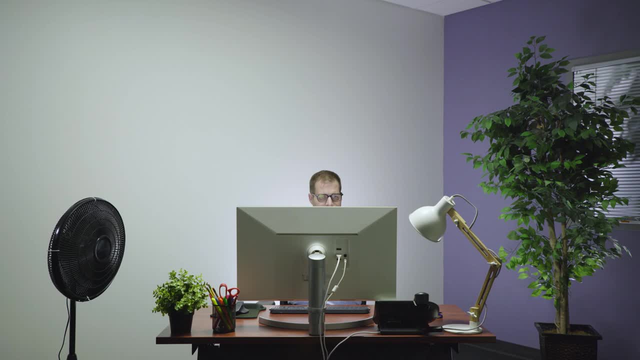 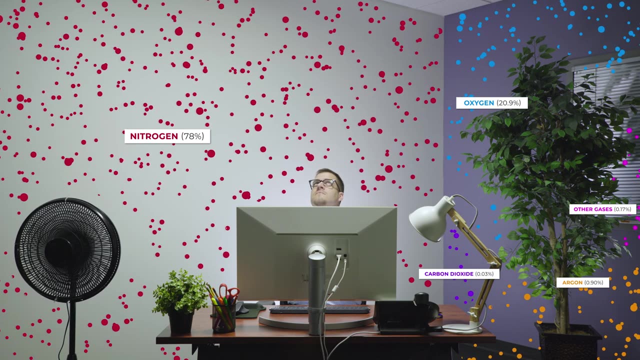 those particles. Remember earlier when we said that the air we breathe is typically a mix of gases like nitrogen, oxygen and carbon dioxide, among others. Whenever we inhale this air, our body acts as a filtration system and we exhale the 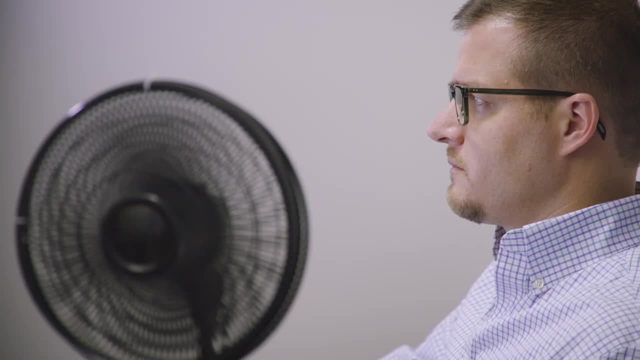 gases that we don't need, like carbon dioxide. If we need to breathe, we need to breathe. If we need to breathe, we need to breathe. If we take a pollutant and throw it into the air's composition, such as radon or asbestos. 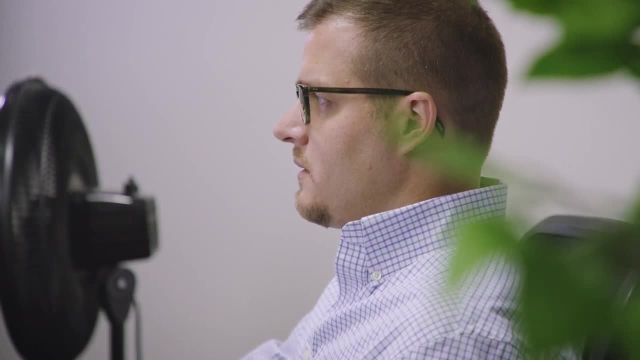 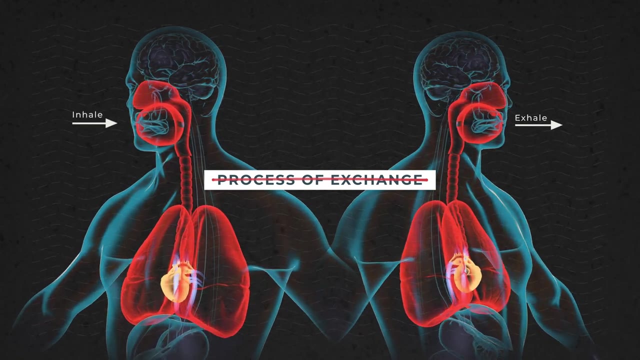 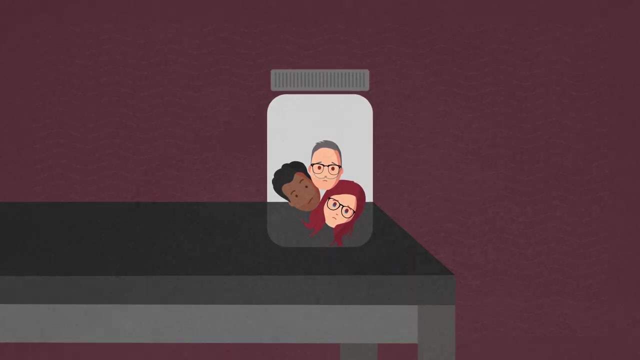 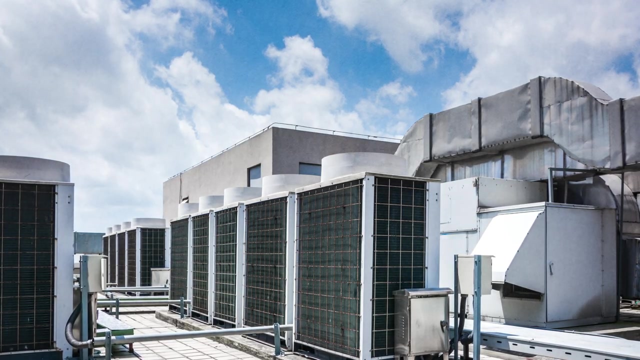 fibers, then we are ingesting a substance that our body cannot naturally filter. This is when the human reflex of breathing no longer becomes a process of exchange. In essence, we become storage vessels for contaminants and are left to deal with the consequences. When it comes to facility management, the basic upkeep of an HVAC system is 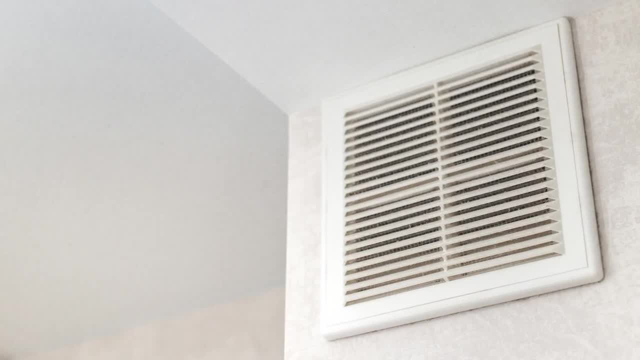 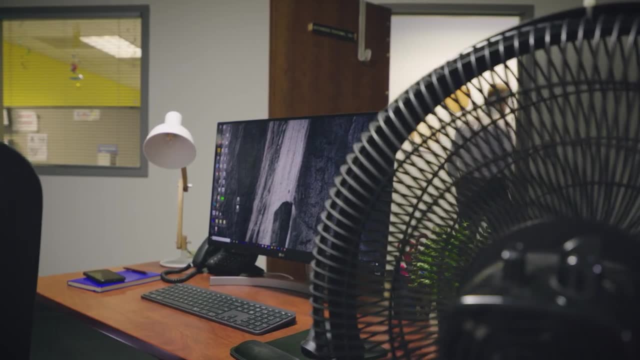 often prioritized over the quality of the air that flows through it. Additionally, since the effects of air pollutants are felt and not seen, it can be easy to act like they aren't there. In the face of the recent pandemic, we can no longer take this approach. 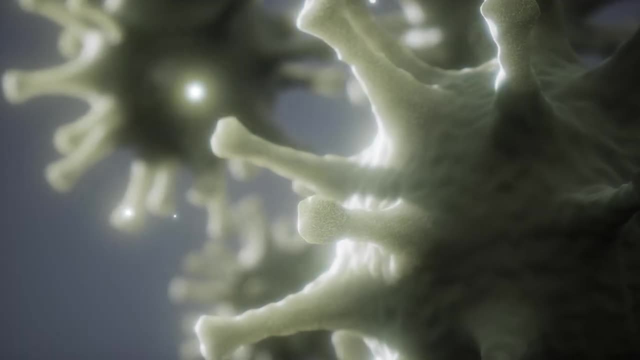 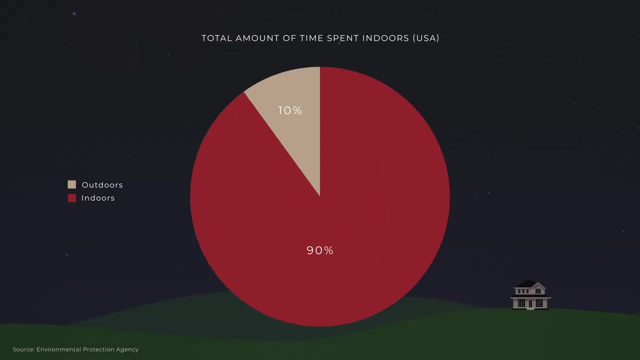 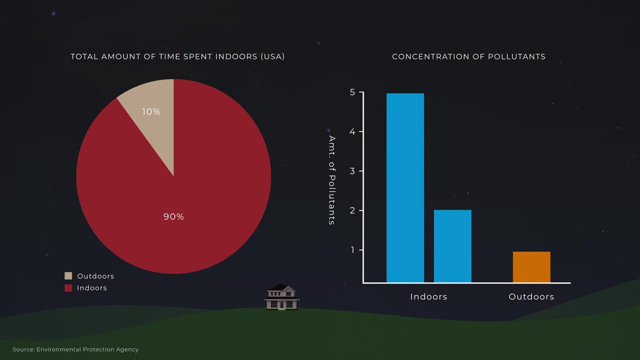 IAQ means the difference between the spread of germs, bacteria and disease, and, in some cases, life and death. According to the EPA, Americans on average spend approximately 90 percent of their time indoors, where the concentrations of some pollutants are often two to five times higher.